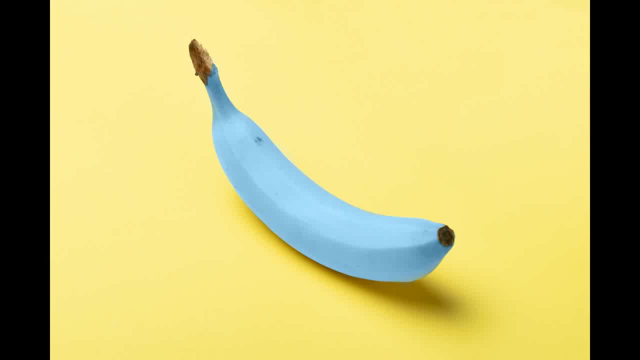 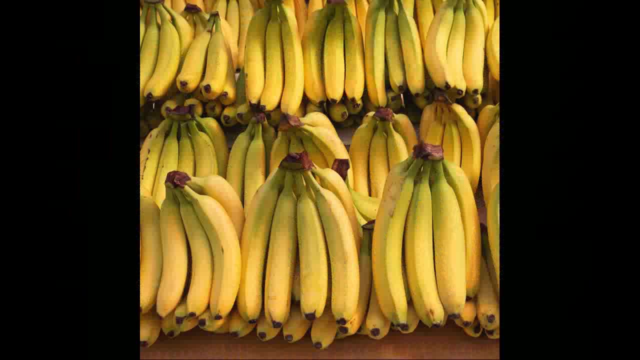 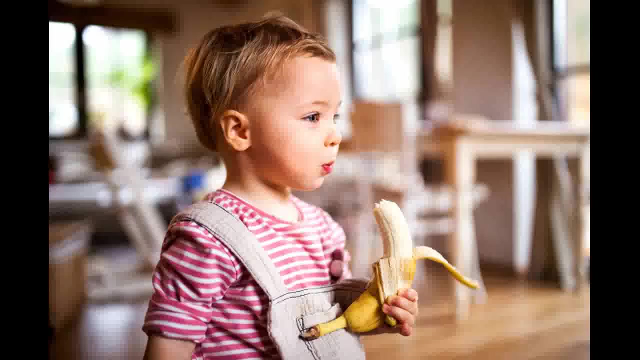 Originating from Southeast Asia, bananas are believed to have been first domesticated in Papua New Guinea. These early bananas were quite different from what we eat today, containing large seeds and having a starchy, less sweet flavor. Over centuries of cultivation, they were transformed into the seedless sweet fruits we know and love. 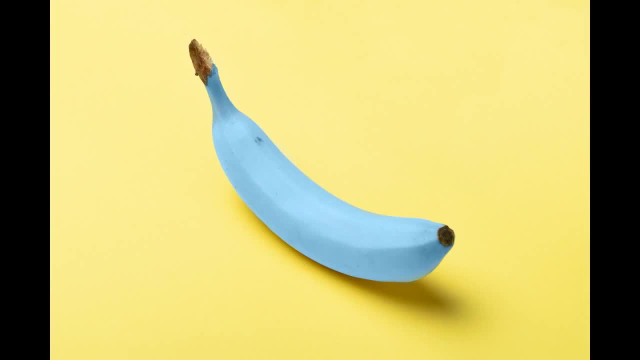 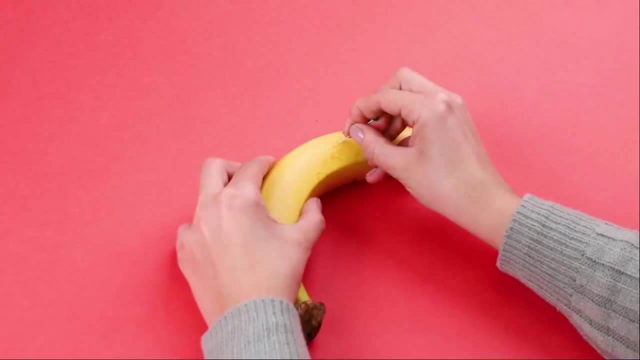 The clone conspiracy Unveiling the reality of modern bananasA startling fact about modern bananas is that the vast majority are clones of each other. The most common variety, the Cavendish, is genetically identical across the globe. This lack of genetic diversity makes bananas 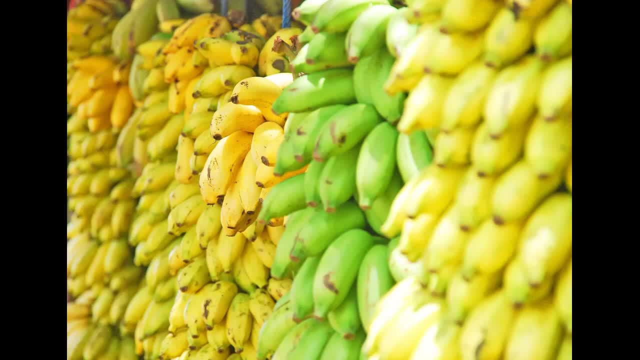 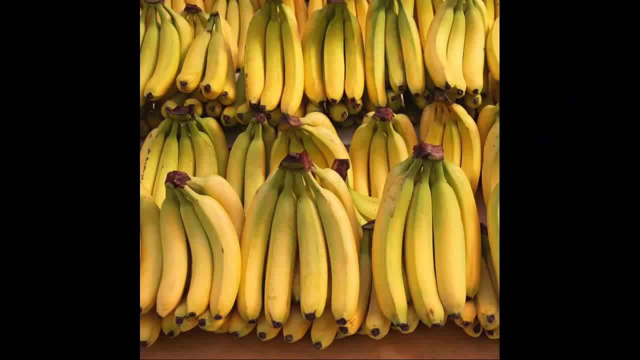 extremely vulnerable to diseases. In the 1950s the Gros Michel, then the dominant banana variety, was almost wiped out by a fungal disease called Panama disease. The Cavendish replaced it because of its resistance to that particular strain. But now, 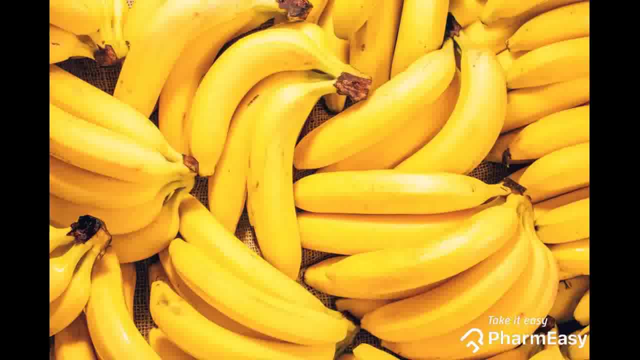 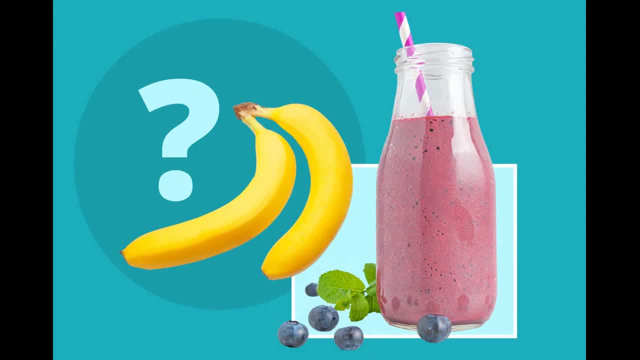 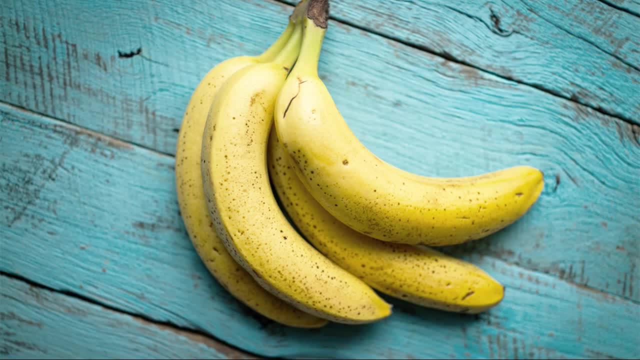 a new strain threatens the Cavendish, highlighting the risks of this genetic uniformity. The environmental impact Understanding bananas' ecological footprintThe cultivation of bananas has significant environmental implications. Large-scale banana farming often leads to deforestation, soil erosion and water pollution. 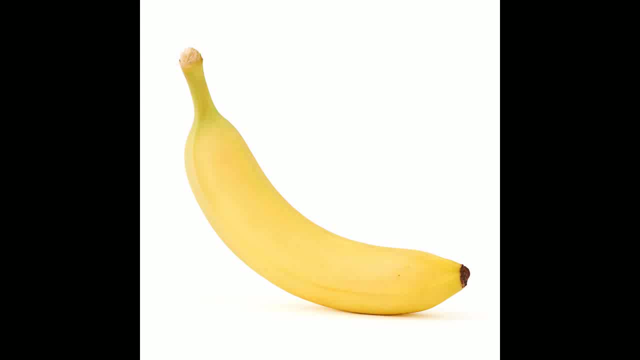 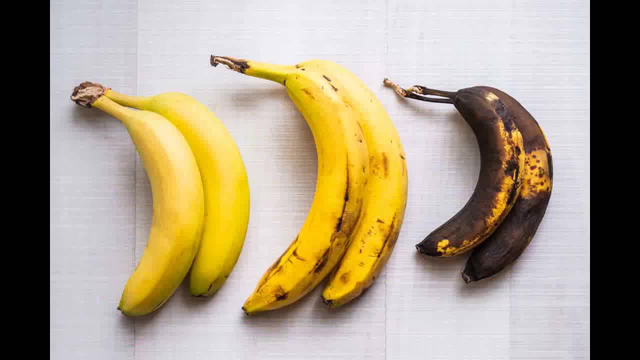 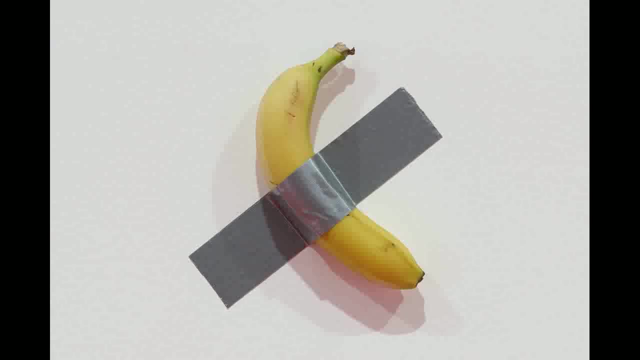 Due to pesticide use. These plantations also consume vast amounts of water, impacting local ecosystems and communities. Additionally, the transportation of bananas across the globe contributes to carbon emissions. Sustainable farming practices and organic bananas are becoming more popular, offering a more environmentally friendly option for consumers. 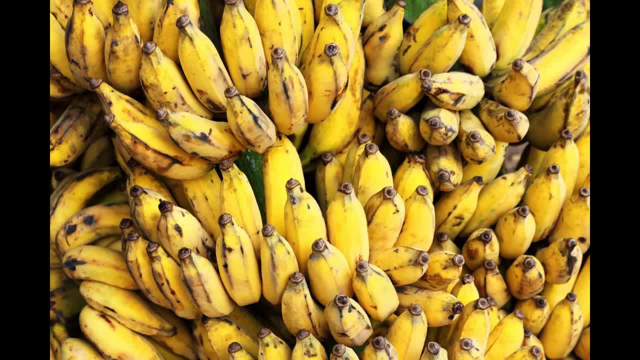 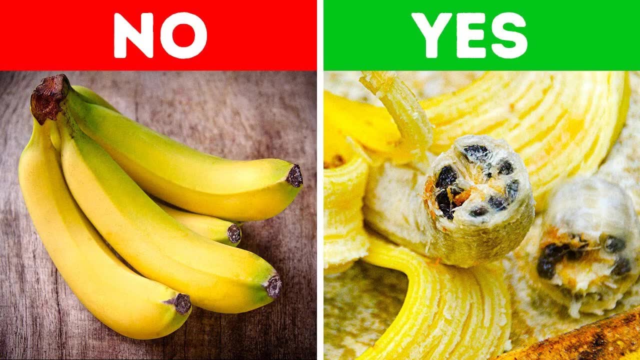 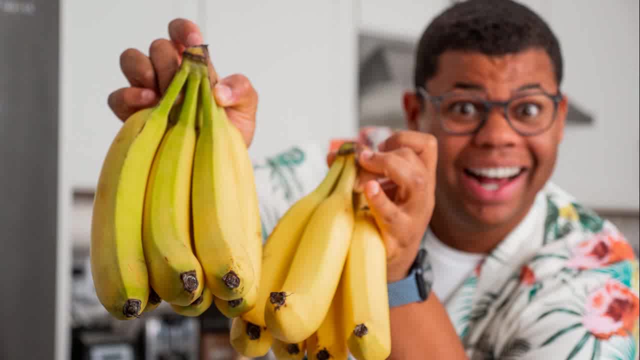 Health myths. debunked The nutritional misconceptions about bananasThere are several myths regarding the health benefits of bananas. While they are a good source of potassium, fiber and vitamin C, the belief that they are exceptionally higher in potassium than other fruits is misleading. In fact, many other fruits and vegetables, like avocados and sweet 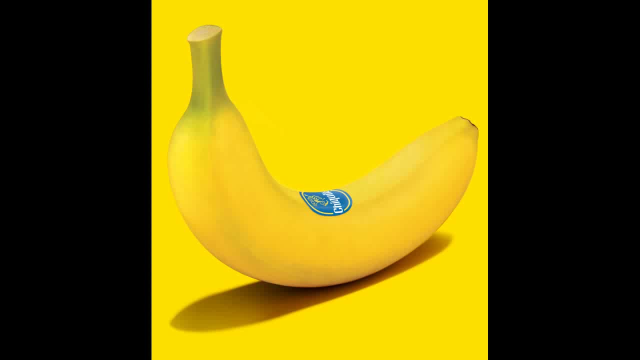 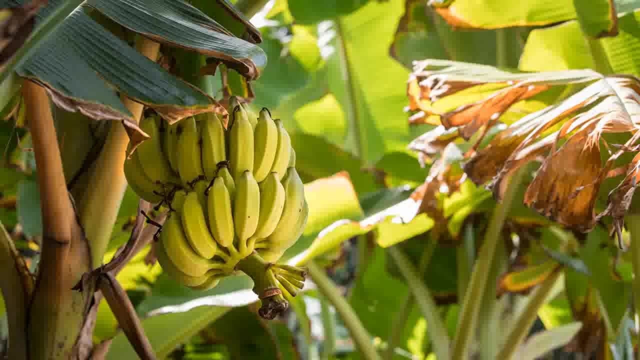 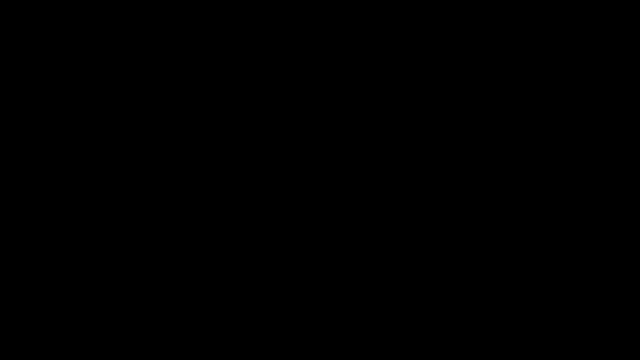 potatoes contain more potassium. Bananas also have a high sugar content, which can be a concern for individuals with certain dietary restrictions. However, they remain a healthy, nutrient-rich snack when consumed in moderation. The future of bananas: Scientific innovations and challengesThe future of 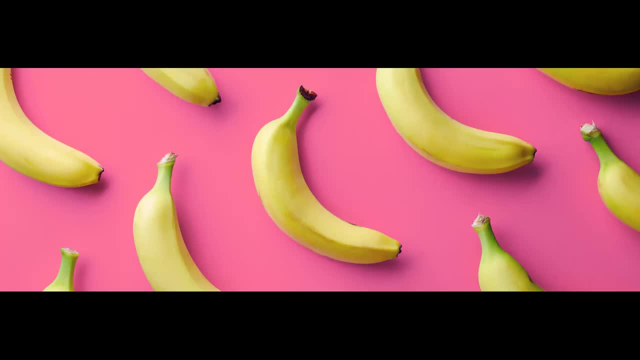 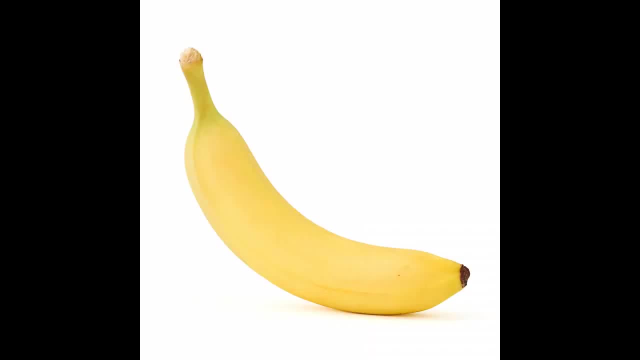 bananas is being developed. The future of bananas is being developed. The future of bananas is being shaped by scientific advancements and challenges. Researchers are working on developing new varieties that are resistant to diseases and pests. hoping to prevent a potential banana crisis, Genetic modification and cross-breeding techniques are being explored as solutions.